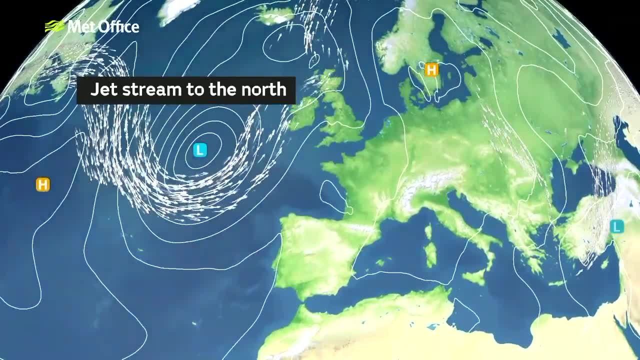 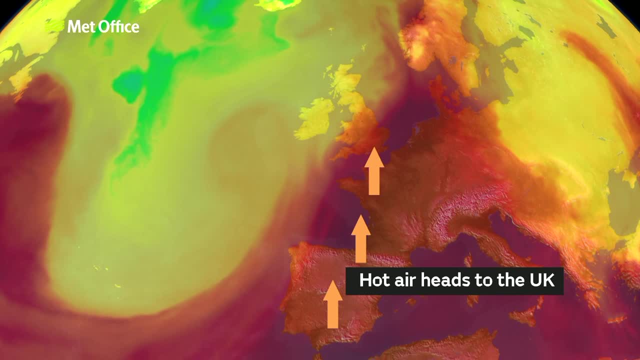 heat waves in the UK when high pressure develops over the UK or Europe, let in by the fact that the jet stream will have moved further north during the summer months, And when these conditions persist for a period of time, it can bring dry, settled, very sunny weather. 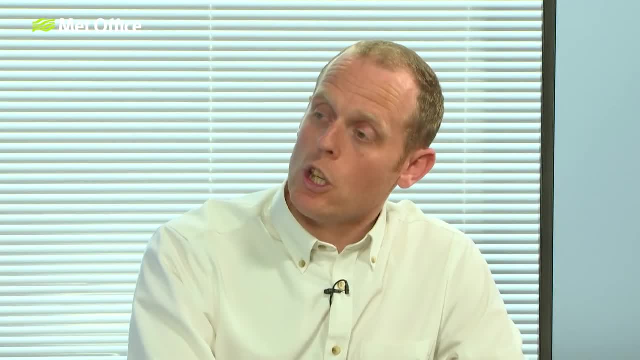 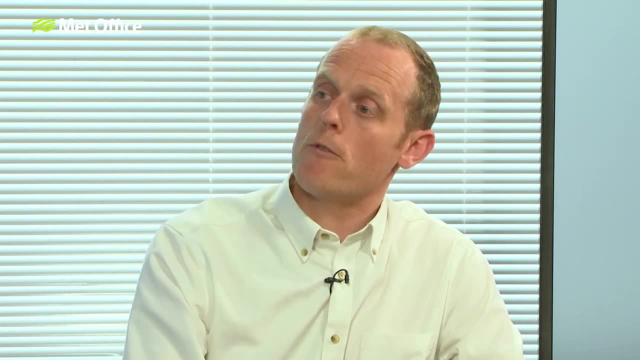 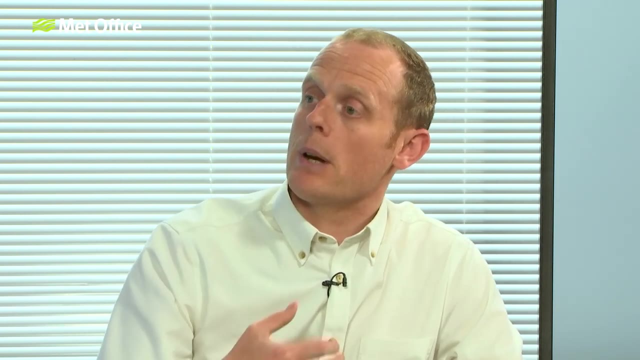 and allowing higher temperatures to build, And here in the UK the hottest temperatures that we tend to get will originate with air that has come from Southern Europe or North Africa. These might be referred to as Spanish plume events, And they bring the hottest. 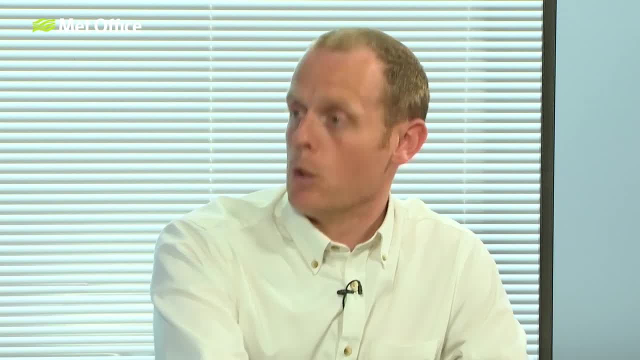 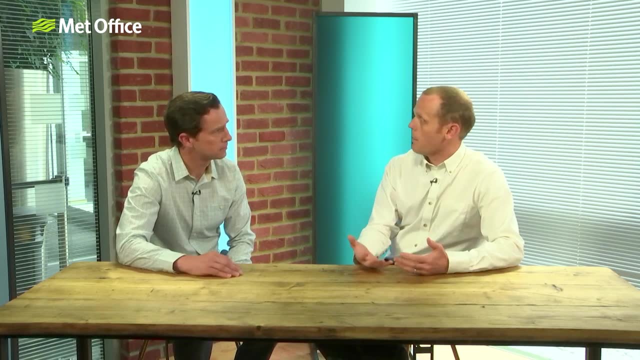 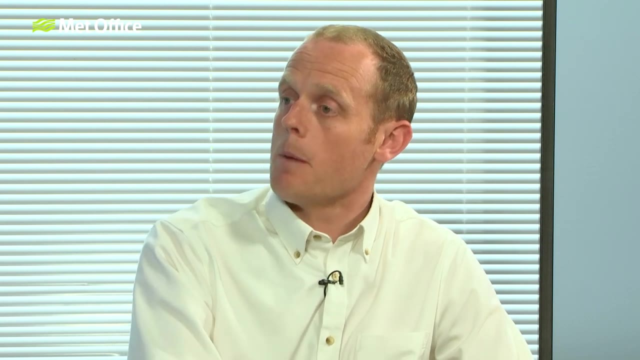 air over the UK, And that's often when we see the records being broken. And is there a link between UK heat waves and climate change? Well, what climate change means is that when we get the right weather conditions for heat waves and that hot air, climate change can make it more likely that we'll 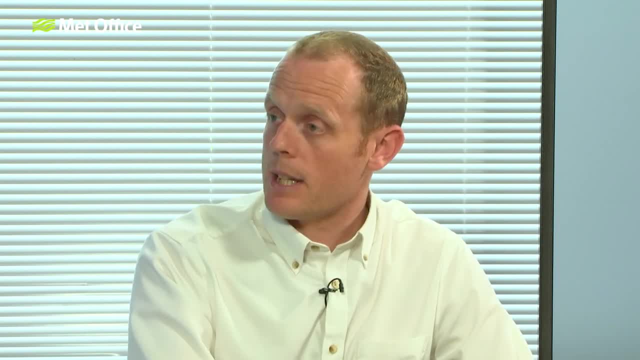 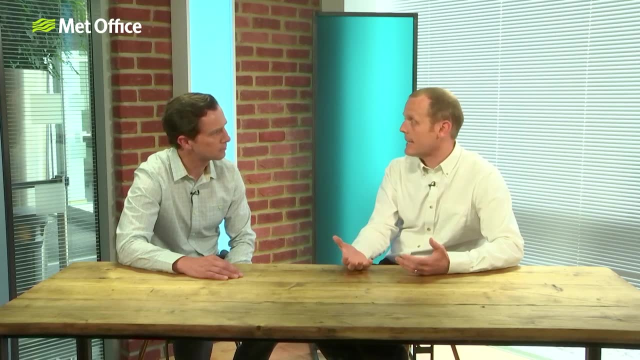 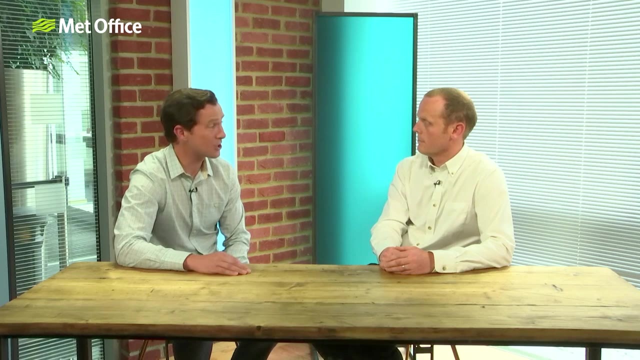 see sort of more extreme temperatures. The global temperature has warmed by about as agree compared to pre-industrial times And this means that actually we are seeing more hot days and more heat waves, globally speaking, than we were before. We're seeing extreme temperatures this week. Mark across the UK Is this week's heat wave. 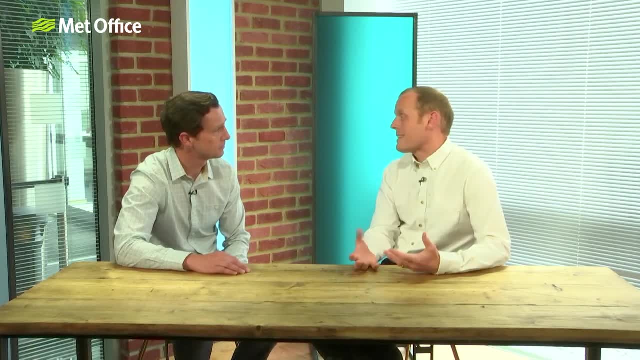 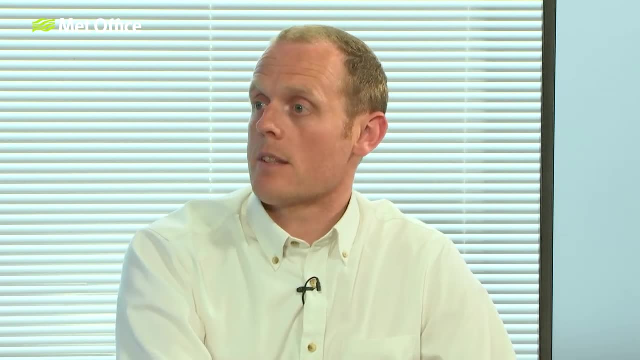 to do with climate change. Well, in some sense, that's not quite the right question. So what we look at in climate science is how climate change has influenced the likelihood or the risk of a particular event occurring, And that analysis can take a bit of time, And we need to do that. 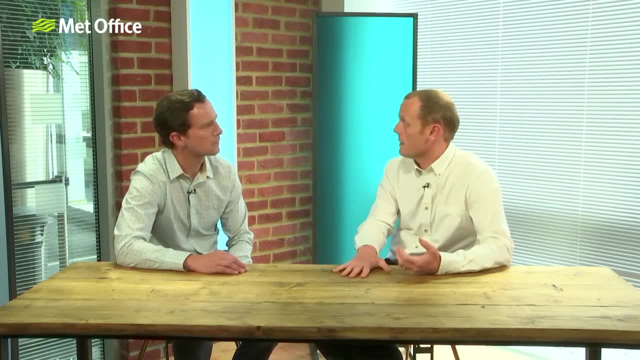 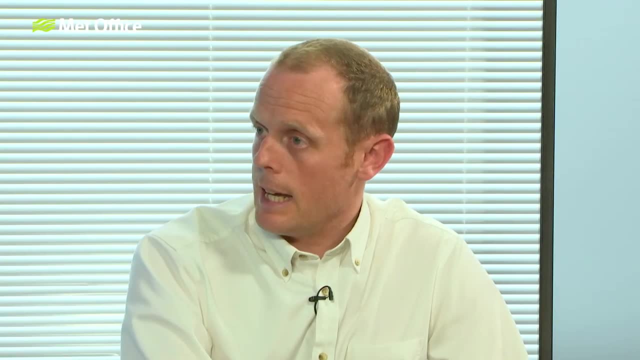 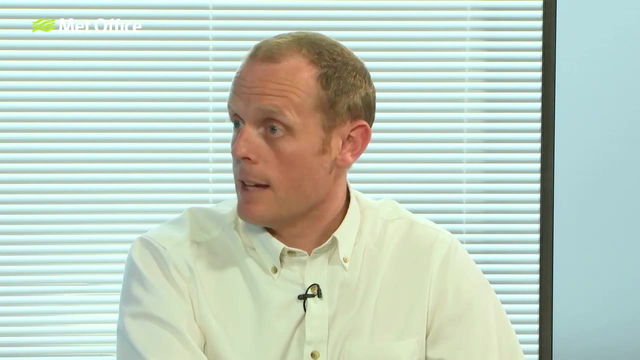 carefully after the event, using statistics, Statistical analysis, observations and climate models. But what we can say in general is that the globe is warming and the UK is warming, And that warming climate is associated with increased frequency of hot days and heat waves across the world. 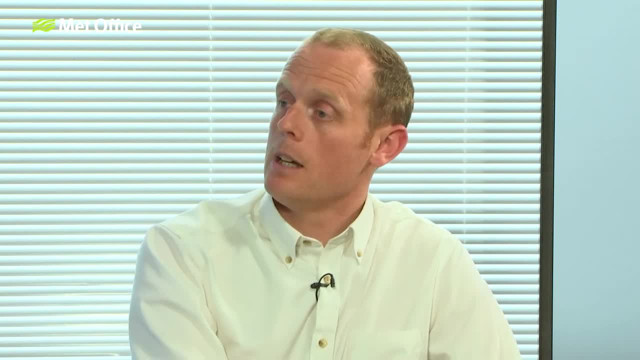 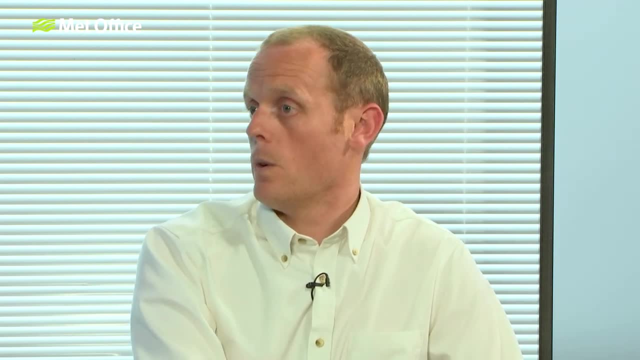 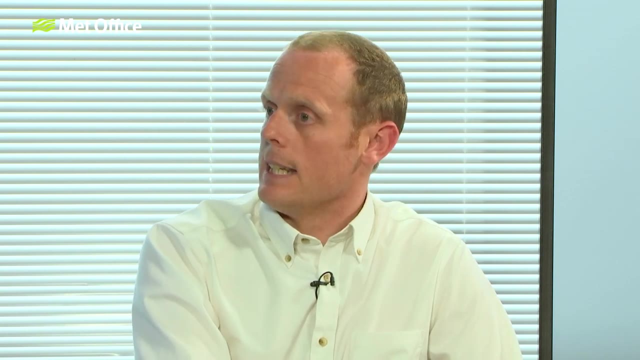 And an analysis that was conducted after the record-breaking summer of 2018 showed that that summer, that heat wave was 30 times more likely due to man-made emissions of greenhouse gases than compared to a world where we hadn't released those greenhouse gases. 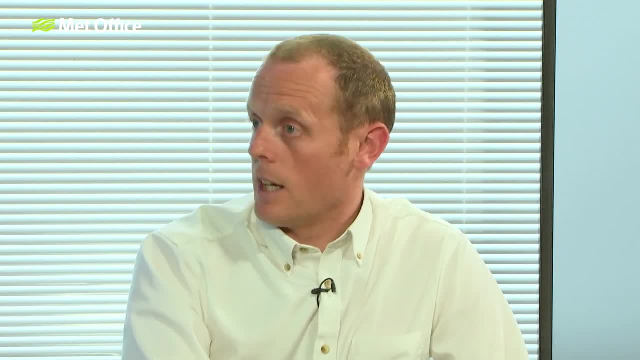 And our projections into the future suggest that summers like that, which are currently quite extreme, might be a fairly typical summer by the 2050s.